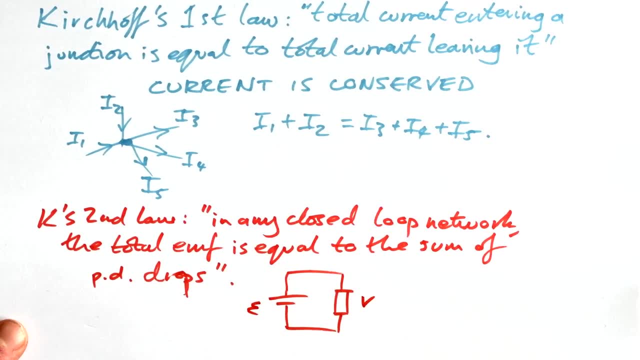 that we can have. We have an EMF here and we have a voltage across here. We know that if this EMF is 6 volts, then the PD drop across. this resistor must also be 6 volts. If we have two resistors in there, again the total PD drops across. both resistors must be 6 volts. 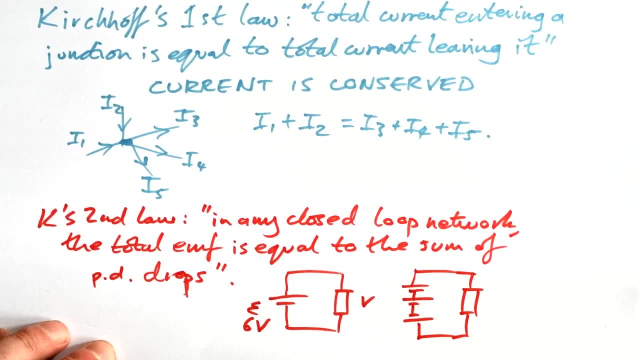 Just be aware that when it comes to EMFs though, batteries and cells do push in a certain direction. So if all of these are 3 volt cells here, what is the total EMF of the circuit? Well, pushing this way, we have 3 volts. pushing this way, we have 3 volts from the cell in the middle. But this 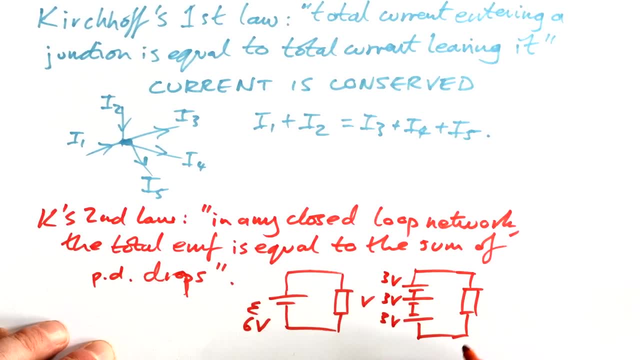 one here is trying to push in the opposite direction. So therefore, actually, the total EMF is just 3 volts, because these two cells are cancelling each other out, as it were. So therefore the PD drop across this resistor also has to be 3 volts. 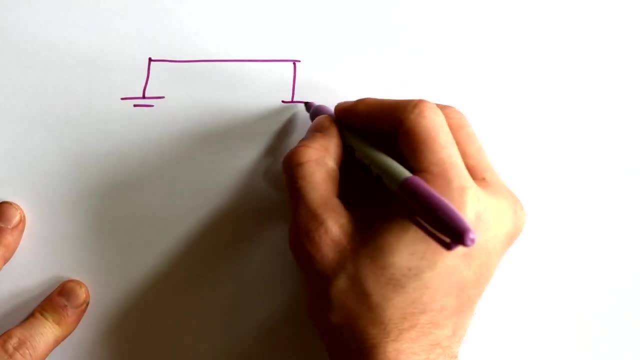 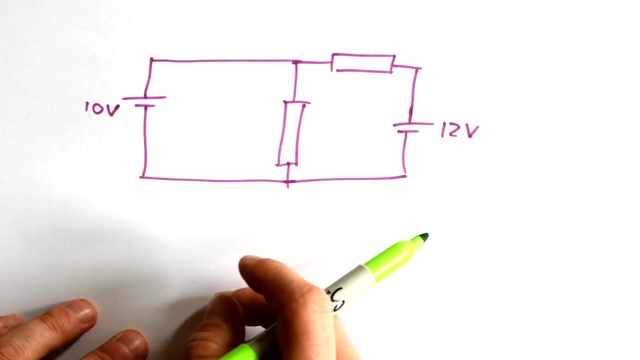 Okay, let's have a look at a more complicated example of how Kirchhoff's second law can be used In this case. we have two EMFs, but they're not in line with each other. as it were, They're part of this branching cell. 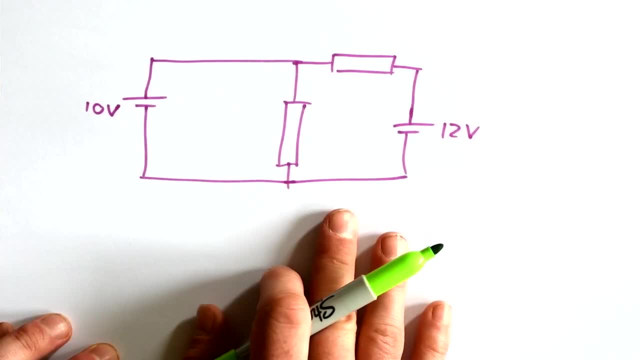 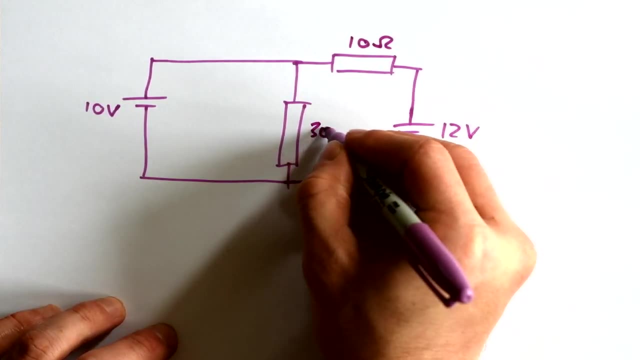 This is the circuit, this parallel circuit, And so this is a very standard case of when we have to use Kirchhoff's second law. We're told the resistance of this resistor is 10 ohms and we're told that this one is 30 ohms. 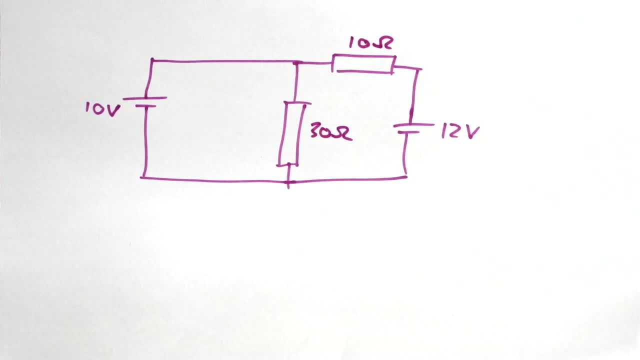 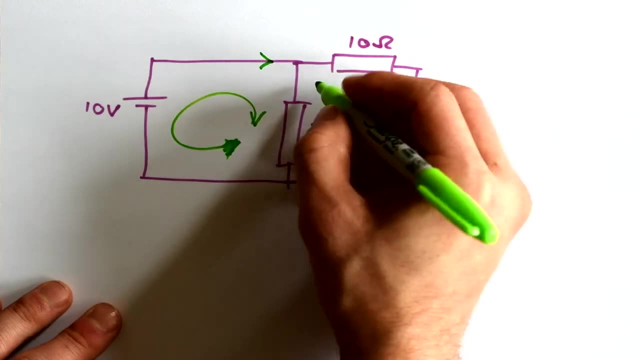 Now, how many loops can you see in this situation? Well, here we have one loop here. Technically, that should be the other way round, because current is flowing this way. We know that current is going to flow in this way and this way. 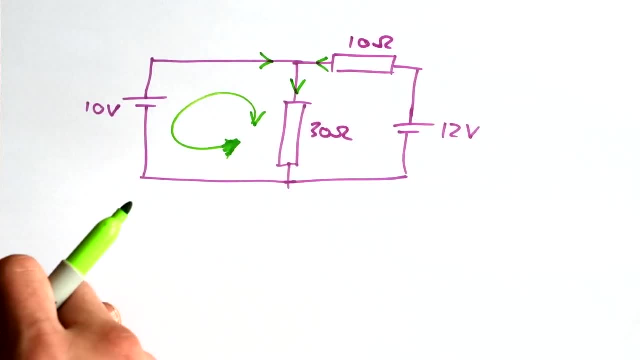 Actually, it's not always obvious which way currents are going to flow. So if you get given questions generally, you will be shown which way the currents are flowing. Okay, we have another loop here as well. It's just a closed loop, so there's one loop. 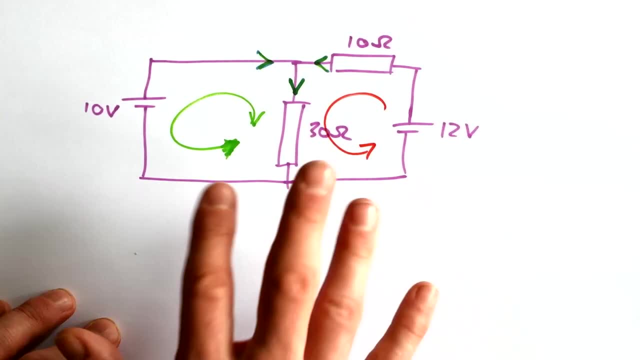 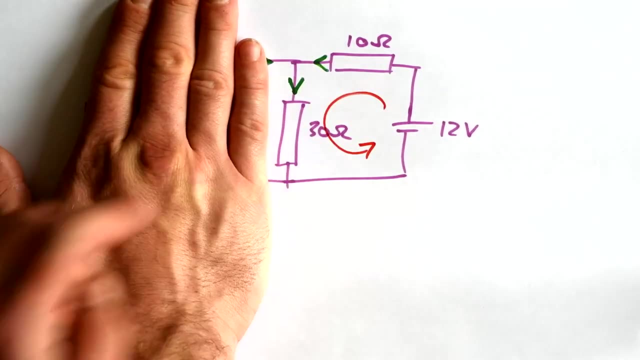 We can literally just forget about that. We have to consider the circuit as a whole, but we can break it into just different loops. There's one loop that's the cell and the resistor, and here's another loop- cell and two resistors. 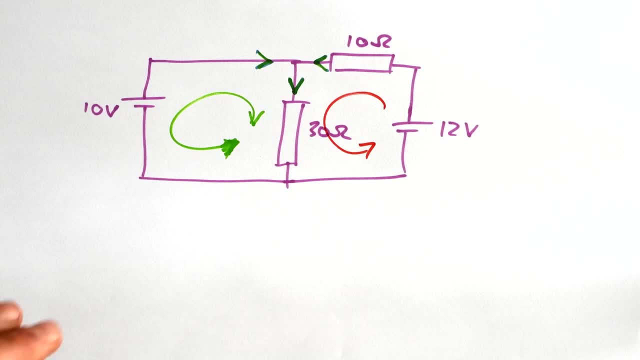 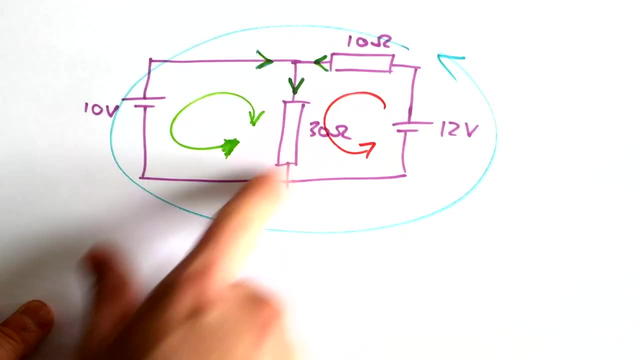 But there is one more loop as well. It's like one of those puzzles: how many squares or triangles can you see? And we have one big loop as well. Now let's try and figure out what the PDs across these resistors are going to be. 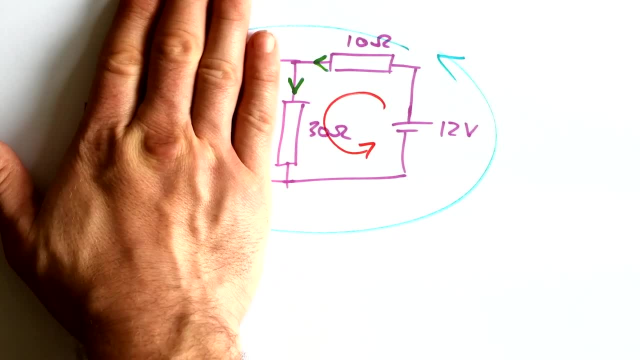 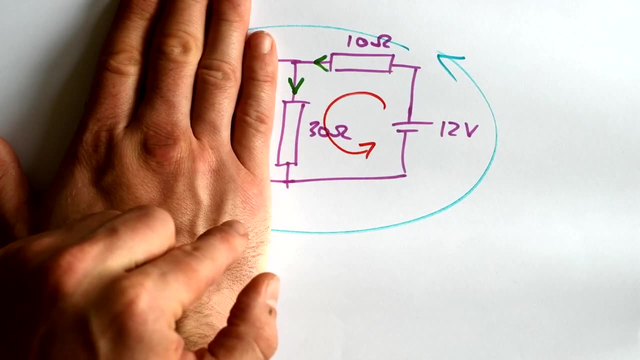 So, at the minute, if we just look at this loop, it seems like we have a potential divider, don't we? Because we have this 12 volts and we have 10 and 30. So if this was just a loop by itself, then we would assume that the voltages would be nine and three. 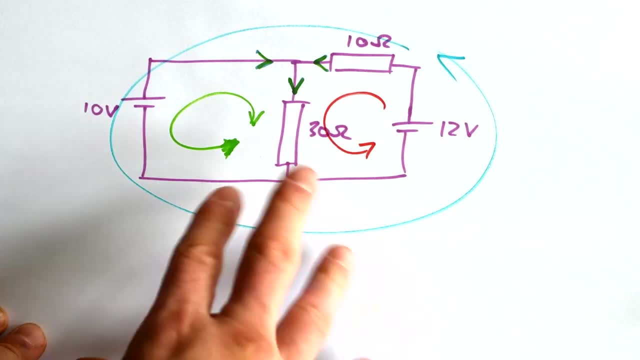 That's just your potential divider equation, But the problem is: is that that's not the only cell involved? We also have this one, And so we can't say that that 12 volts is being split between these two resistors according to their resistors. 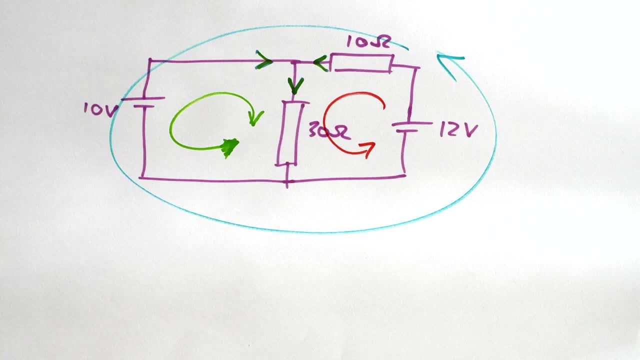 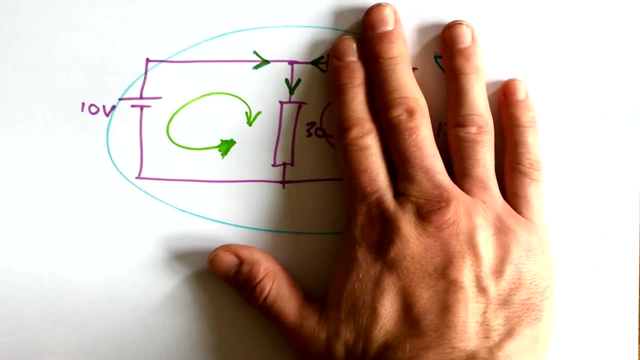 But there is one thing that we know to be true, and that is that we have one loop here where we have a 10 volt battery find cell- it doesn't matter 10 volt EMF- and we have one resistor. We know, therefore, that, due to Kirchhoff's second law, that because we have a 10 volt EMF, 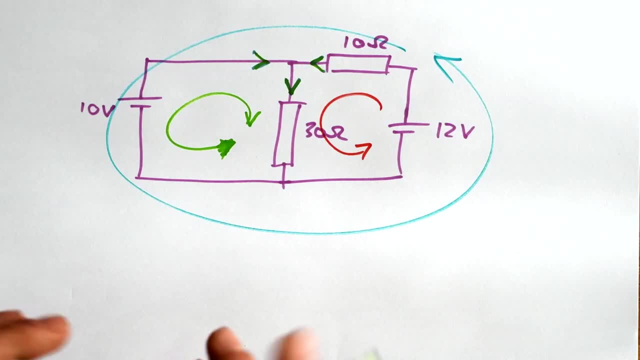 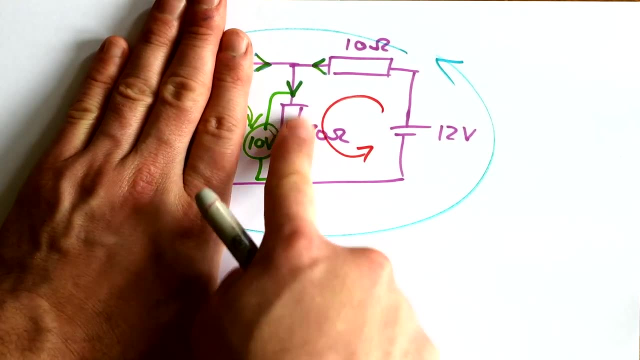 the PD drop across this resistor must be 10 volts. Now we can look at the second loop here We have a 12 volt EMF and we have our two resistors, but we know that it has to be a 10 volt drop across this thing. 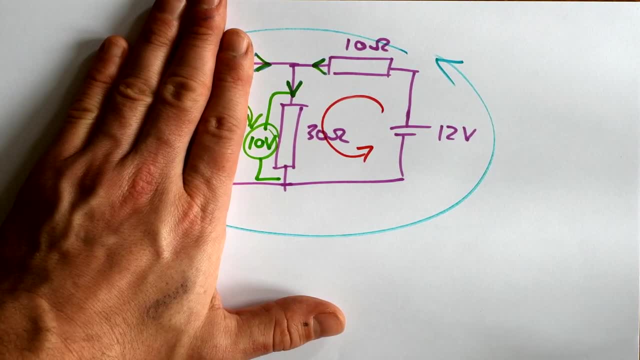 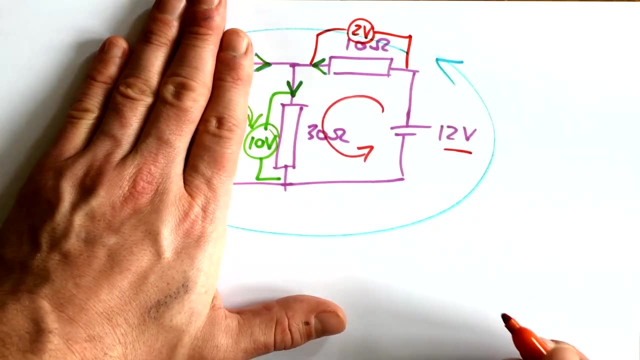 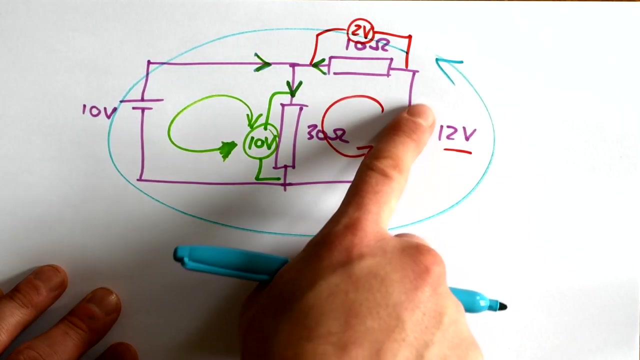 Therefore, now, using our knowledge, that potential has to be divided across two resistors like this. we know, therefore, that this has to be two volts. Let's consider the big loop, forgetting about the resistor in the middle. Here we have a 10 volt battery pushing this way, 12 volt battery pushing this way. 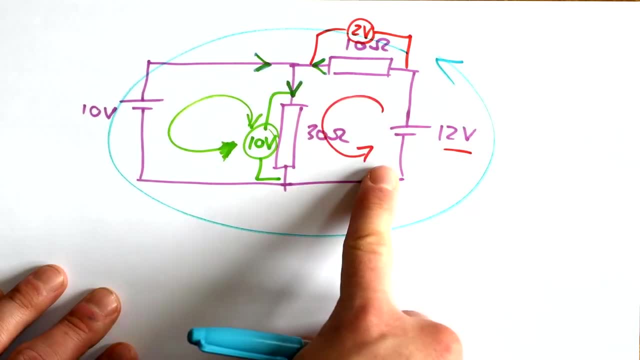 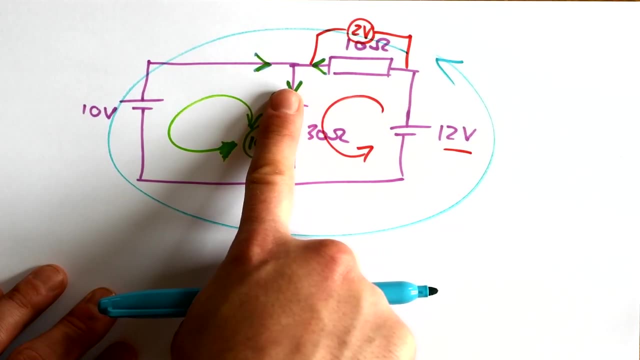 So overall, the total EMF of this big loop is two volts. So therefore, if we're just concerned with this resistor at the top, it has to have a PD drop of two volts, And we've already seen that that is correct. 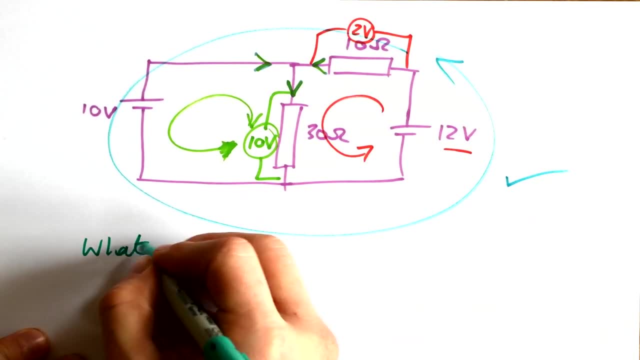 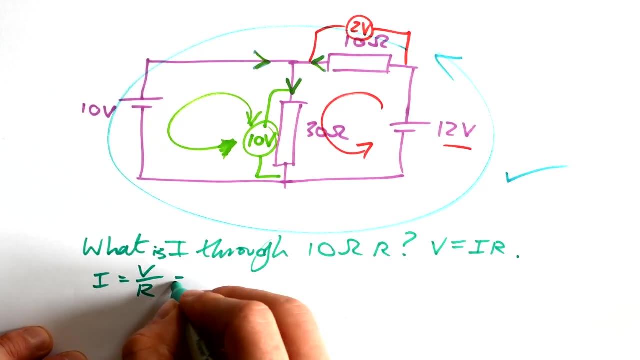 You could then get asked a question like: what is the current through the 10 ohm resistor? Well, we're going to use just V equals IR. I is V over R, But what is the V going to be? Like, we said, it's two volts. 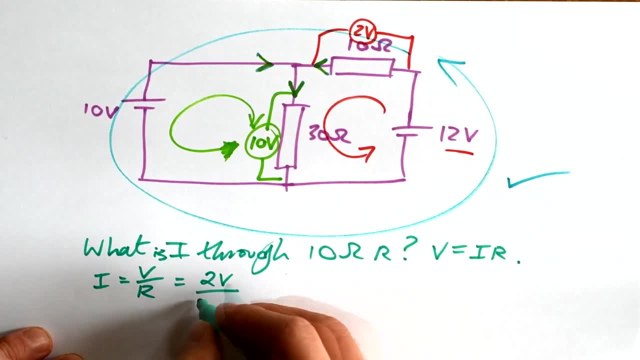 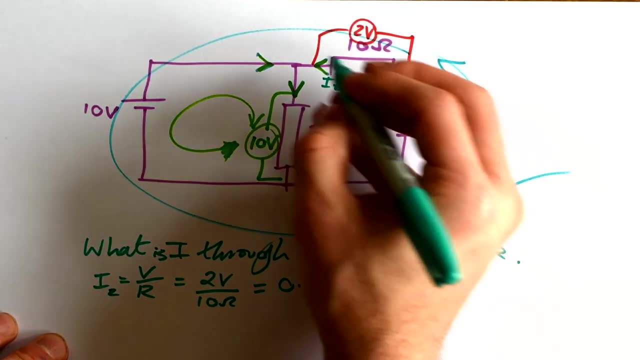 And we could figure that out either from these two loops or just the big loop. Divide that by the 10 ohms and we have 0.2 amps. Tell you what? let's call that current there I2.. Let's call this one I1.. 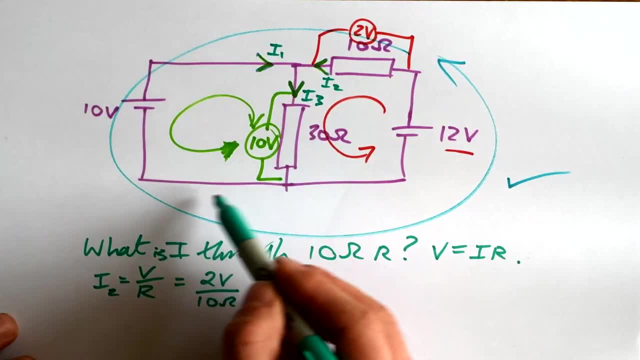 I3. Can we figure out what I1 is straight away? No, we can't, Because we have this branch here and we need to know I3 first. So let's find out I3. Here we have current flowing through this resistor. 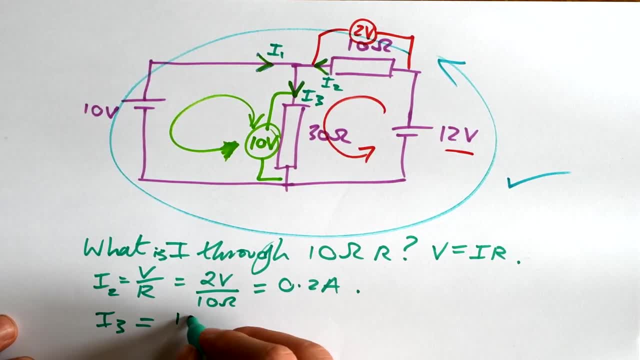 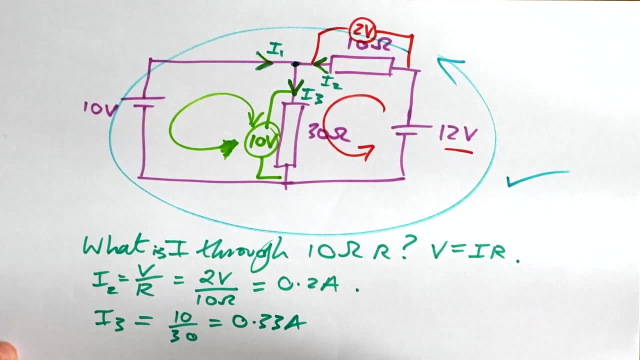 Do we have a voltage? Yes. Do we have a resistance? Yes. So therefore we can just do 10 divided by 30. And so that gives us 0.33 amps. Now we know that at this junction here Kirchhoff's first law has to be satisfied. 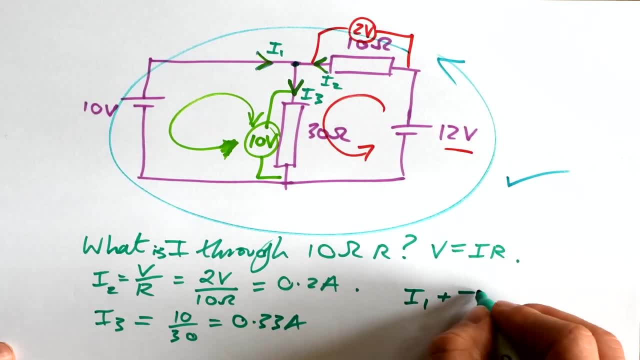 So we can see that I1 and I2 are going in And that has to be equal to I3 coming out. So therefore, if we want to find This current here, the I1, we can say that's going to be I3. take away I2.. 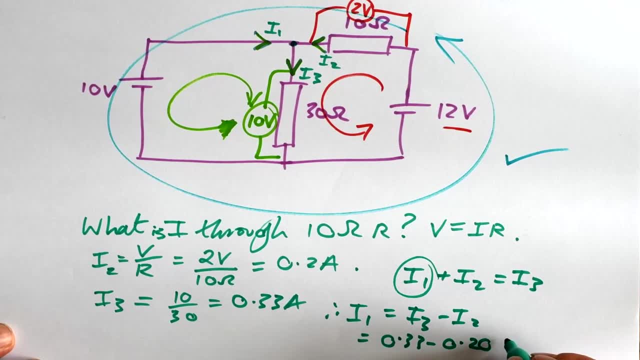 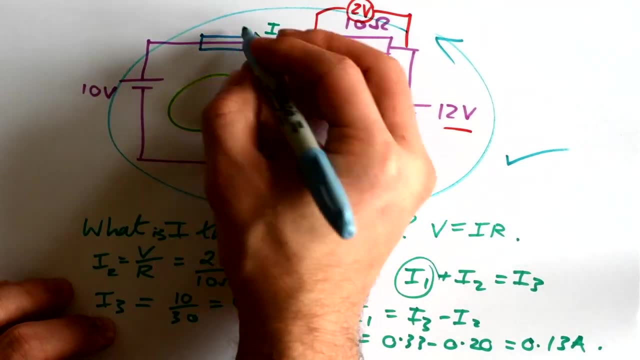 In other words 0.33, take away 0.2. That gives us 0.13 amps. Now it gets complicated when we add in maybe a third resistor. here. Let's call that 10 ohms as well. I'm not going to do any calculations with it because it'll take a while and it's 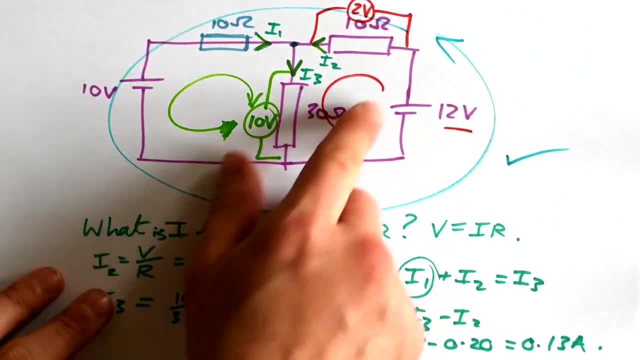 a little bit beyond A level. But the thing is, by adding this one resistor in that changes the whole circuit Again this big loop. here we have a total EMF of 2000.. It'll compute about 22 volts. 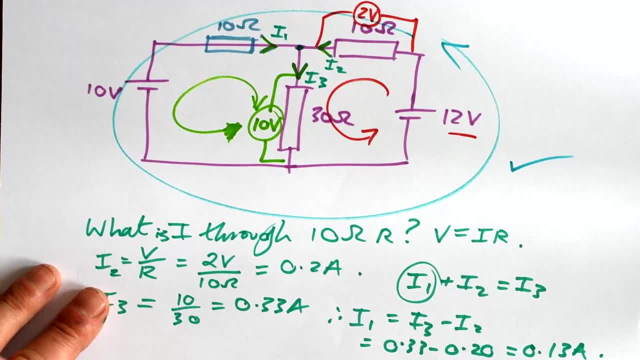 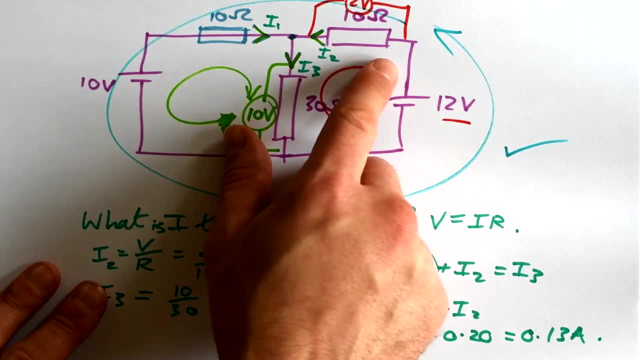 But we can't say that it's just going to be one volt across each of these 10 ohm resistors. It doesn't work like that. But what we can say is that the PD across this resistor here is bound to decrease because that 2 volts now has to be shared somehow across these 2.. 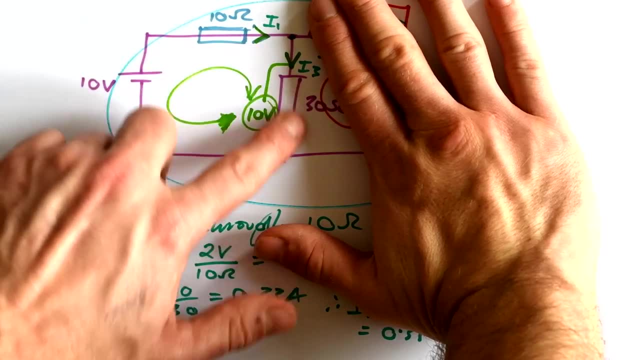 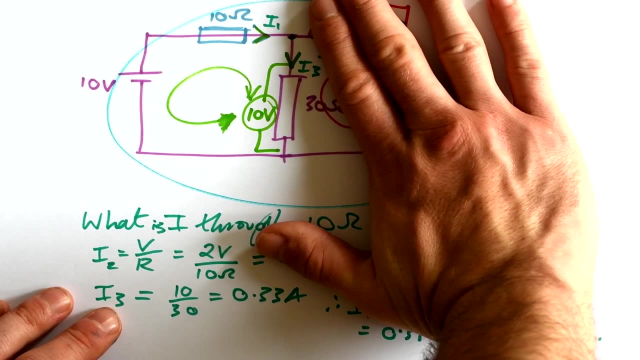 Looking at our first loop over here as well, we now know that this 10 volts has to be shared across the 10 ohm and the 30 ohm resistor. Again, we can't just split that up in a ratio of 3 to 1, because it doesn't work that way. 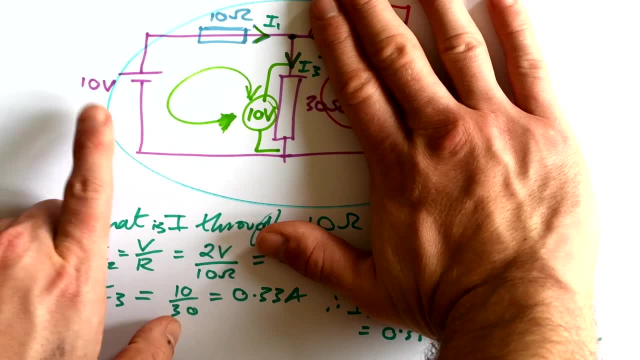 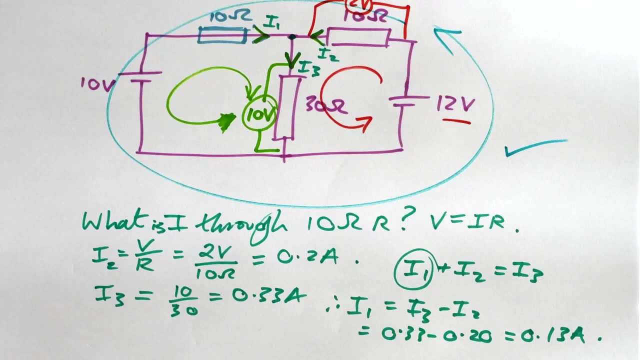 But We do know that the PD across this one is going to be one volt, So is going to drop because, yes, the 10 volts does need to be shared somehow across the 10 ohm and 30 ohm resistor. so there we go. that's a basic look at Kirchhoff's laws. hope you found that. 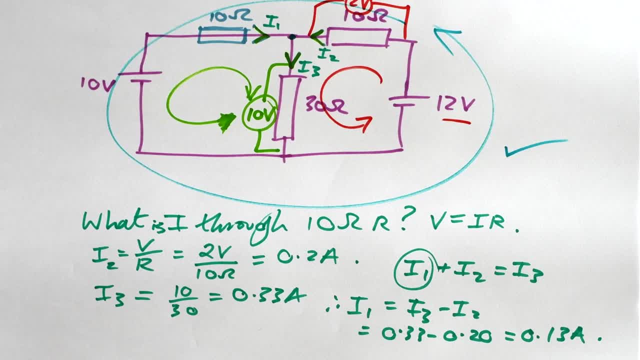 helpful, at least more helpful than the last time. if you did, please leave like. and if you have any suggestions on what I can do next or questions, then please leave them in a comment down below. I'll see you next time.